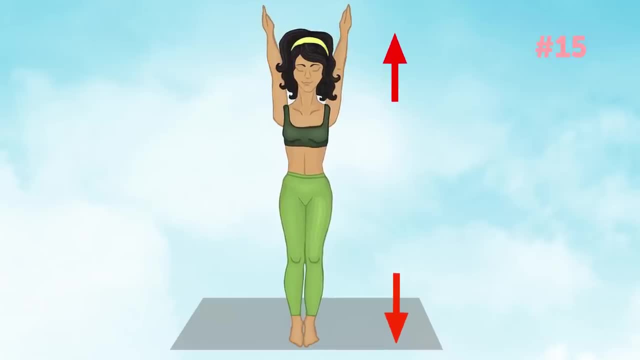 more action. We're going to hold this pose for 30 seconds. Let's go. Tadasana is a great way to improve your posture and, of course, give a proper stretch to your back. A couple more seconds Now. you're ready for all the other exercises. Bhujangasana- cobra pose. 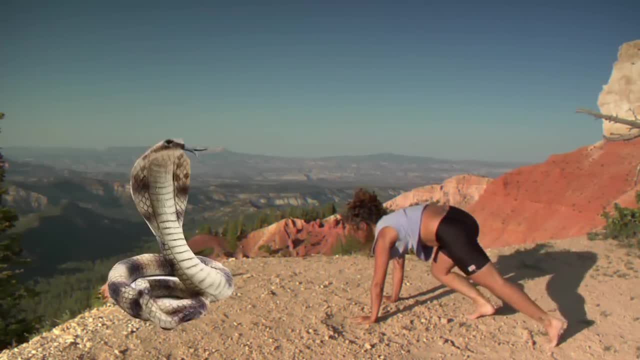 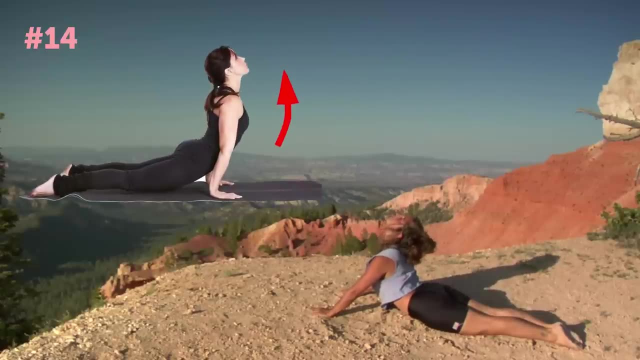 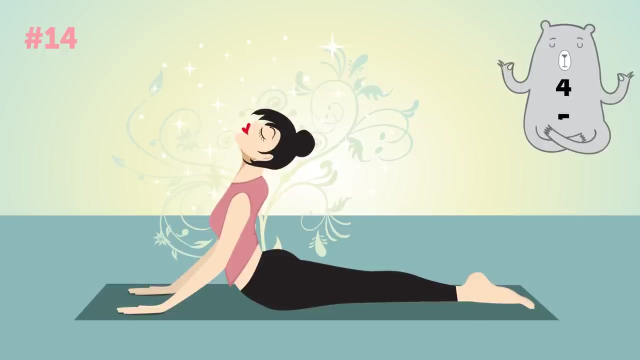 Cobra pose Sounds intriguing. right, First of all, lie face down and spread your arms on the floor. Stretch your legs back and slowly lift up your body. Make sure your pubis and toes form a straight line and touch the floor. Let's try it. Cobra pose has multiple benefits for your body's. 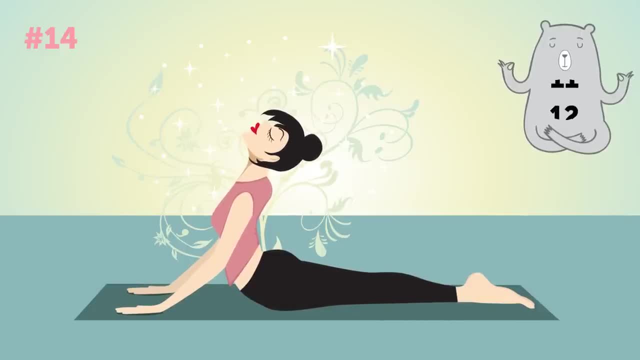 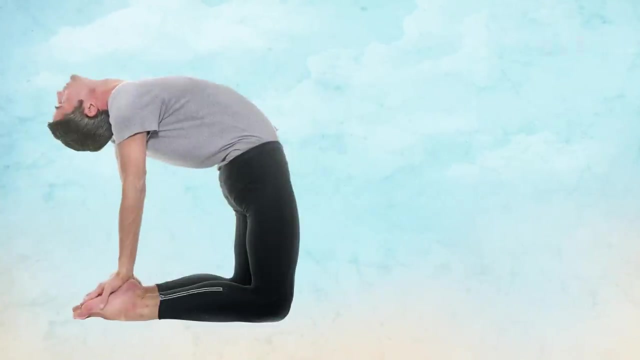 health. It strengthens the spine, firms your buttocks and even helps relieve stress. We're almost done. Good job, Ustrasana camel pose. For this next asana. you have to kneel on the floor and arch your back. 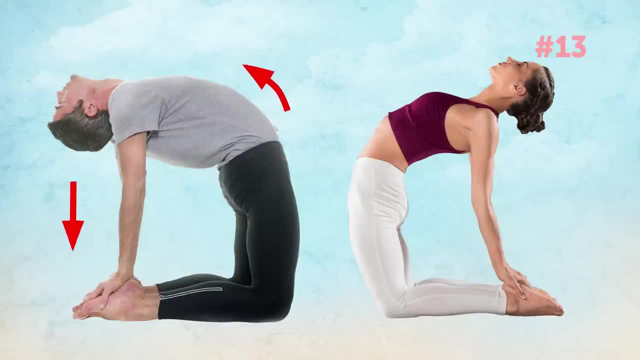 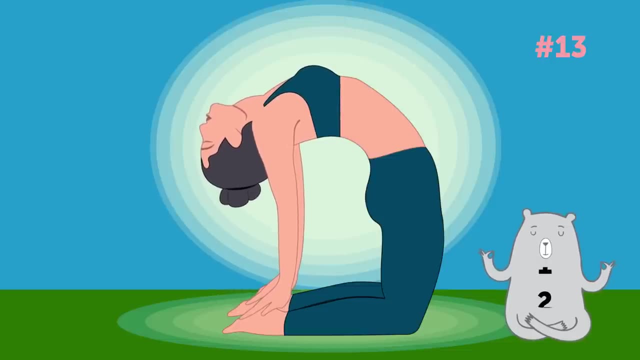 Touch and then hold your heels with your hands. We're going to hold this position for one minute. Time's ticking Ustrasana is a good stretch for your body. It stretches your ankles, thighs, chest and, most importantly for us, abdomen. Moreover, it stimulates the organs of your abdomen. 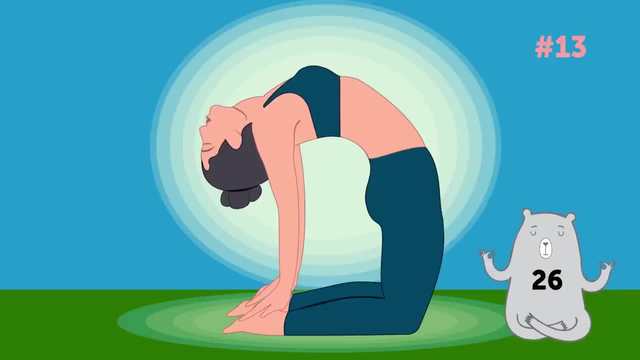 For more exercise. please try to keep your legs straight. For this exercise. you can bend your knees and knees. Toe bar. you should be able to fall down and sit on the floor with your hands. This position is good for you. Toe bar, you can hold your lower back with your hands. 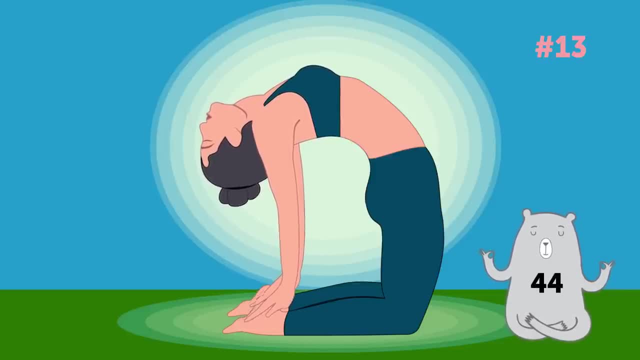 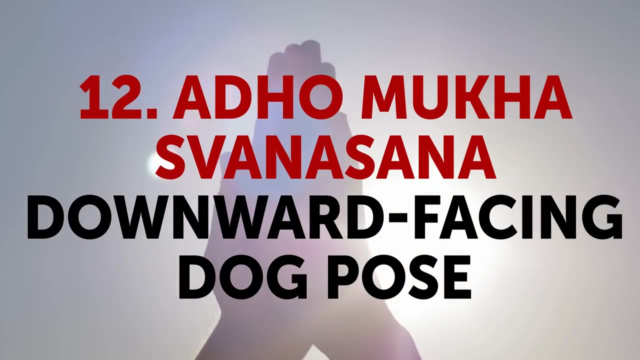 Lower your lower back with your hands. Toe bar. you can hold your lower back with your hands. You can bend your lower back with your hands, And that's it. Take a deep breath and prepare yourself for the next exercise. Adho Mukha Svanasana- Downward Facing Dog Pose. 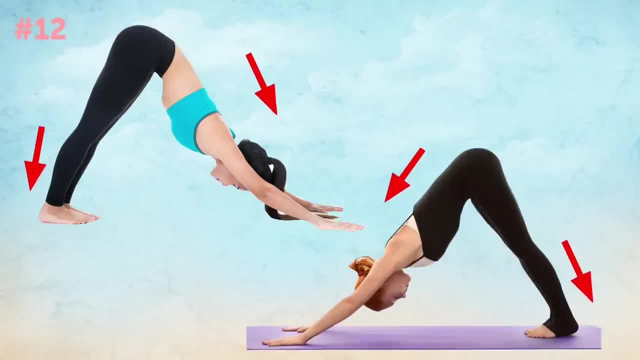 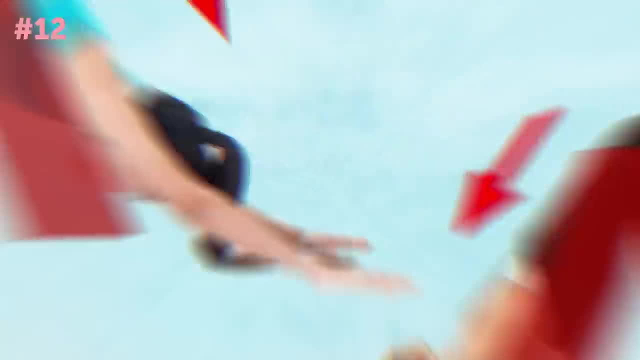 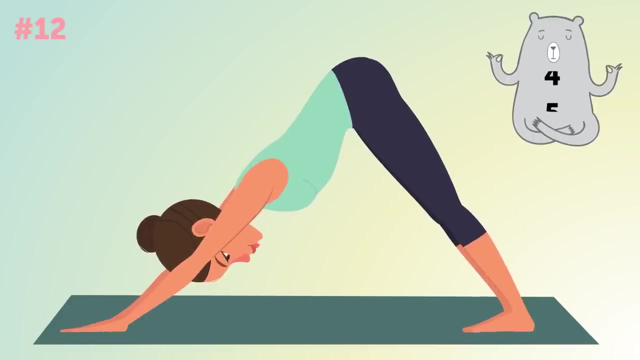 Use your hands and legs to come onto the floor. Then lift your bottom to form a 90-degree angle with your body. Basically, your body should form an upside-down V-shape. We're going to hold this pose for one minute. Let's go. 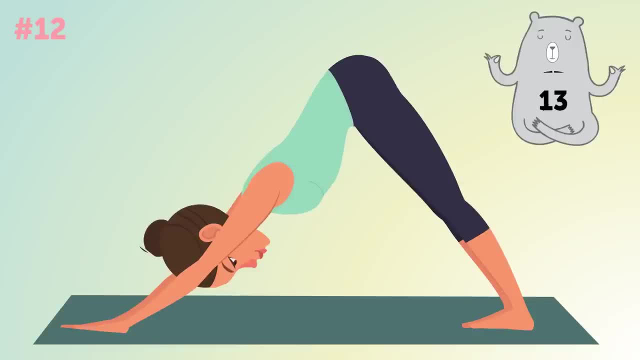 The Downward Facing Dog Pose is one of the sun salutation poses. It helps to both balance the body and work the abs. Additionally, this pose helps relieve stress and mild depression while energizing the body. If you like to sit inAsht Seven Tens with me, talk to me about what you wouldrayshould. 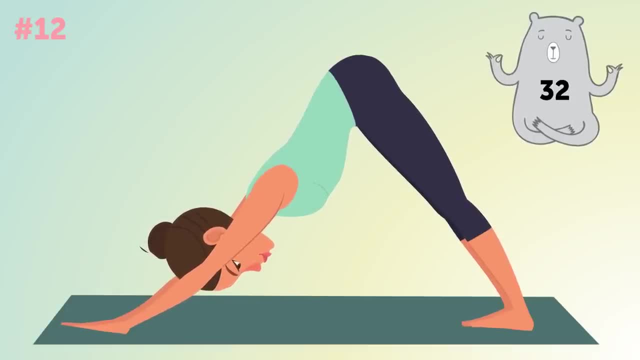 do next, Or you can leave a comment below. You can subscribe to my YouTube channel and follow me on Instagram. Thanks, When doing this pose, mind the back muscles. How are you doing Time's up? Vashisthasana side plank pose. 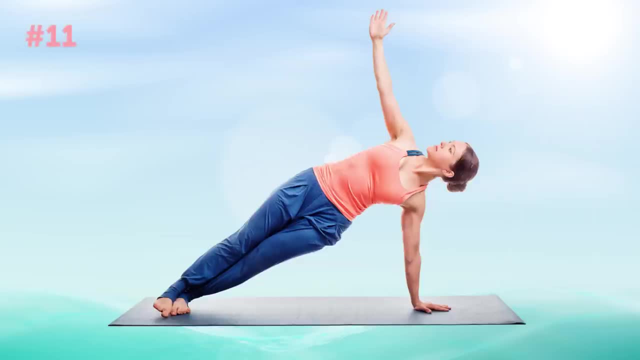 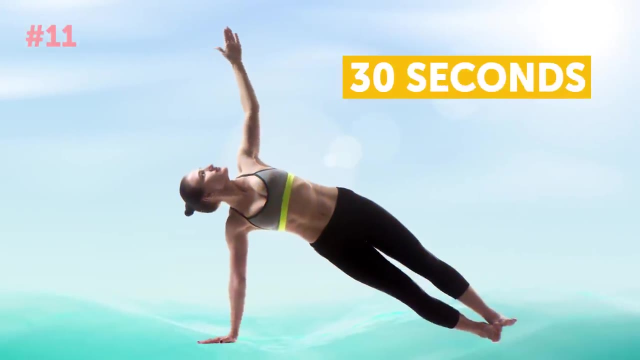 Shift your left or right foot and tilt your body accordingly, either to the right or left side. Raise the opposite arm in the air. Let's hold this pose for 30 seconds and then return to the previous downward-facing dog pose for an additional 10 seconds. 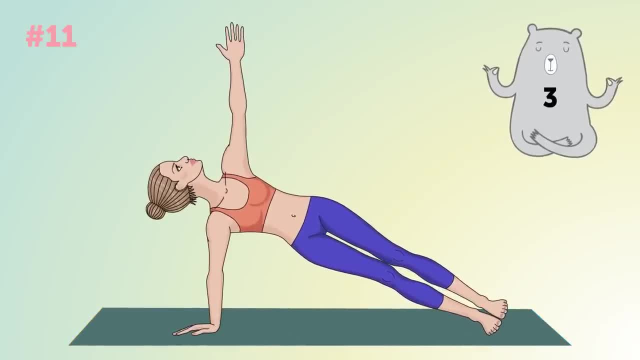 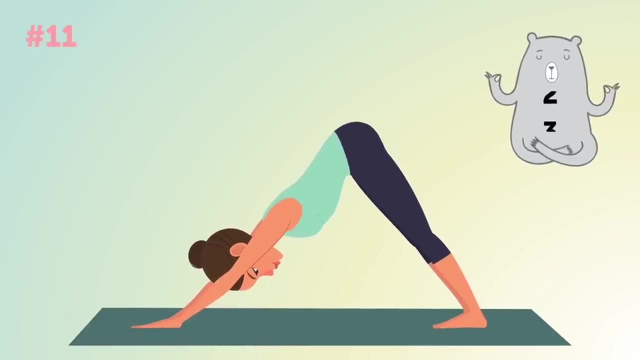 Go. Side plank pose stretches your belly, arms and legs and improves the sense of balance. Good, Now slowly return from side plank To downward-facing dog pose. Stay in it for 10 seconds. Great Pachimottanasana seated. Seated forward- bend pose. To do this pose, you have to stretch your body towards your feet as you exhale and hug your feet with your hands. Nice and simple. Let's try to hold this pose for one minute. This pose, again, is a miracle for stretching your spine, shoulders and tummy. 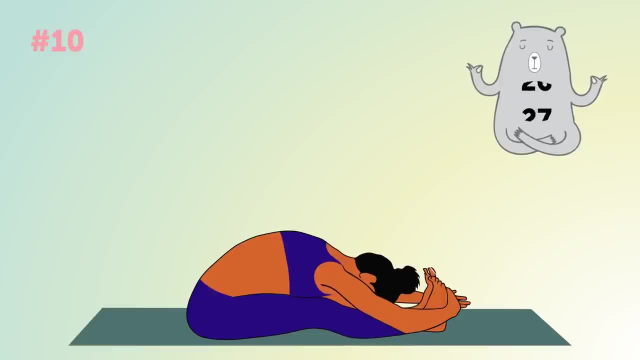 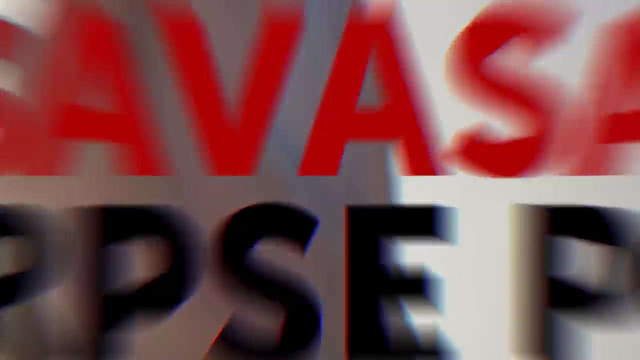 It also improves digestion and stimulates important organs. 30 more seconds, You're doing great. Hold it Stop. Time for the next asana, Savasana corpse pose. Savasana is a relaxation pose. All you have to do is lie flat on the floor. 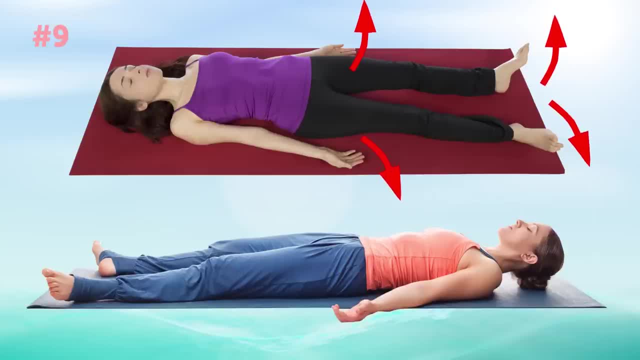 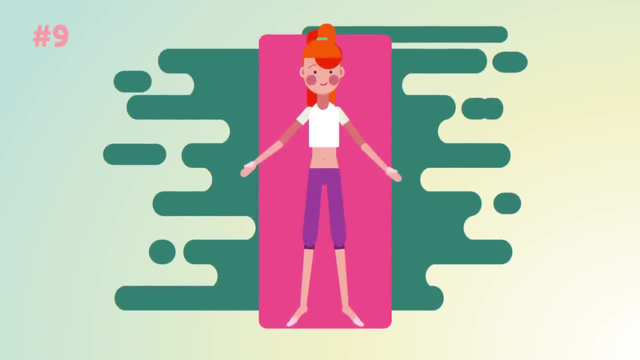 Place your legs so that they're comfortable And you're ready to go comfortably apart and place your arms along the body. breathe slowly and try to focus on yourself and your body. one minute starts now. despite its simple appearance, corpse pose is believed to be the most difficult one. 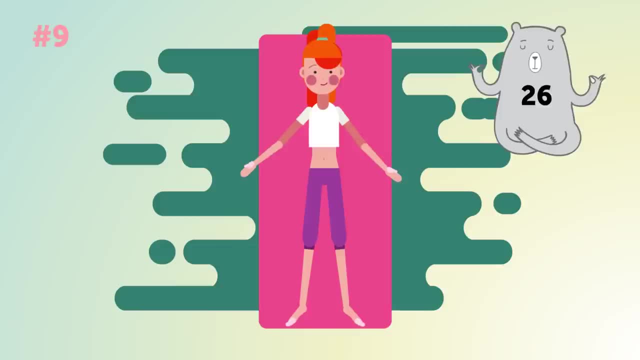 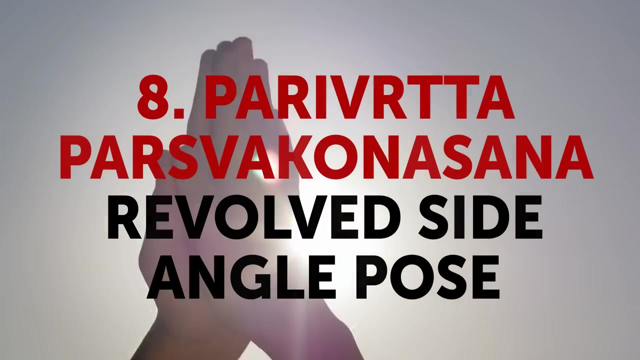 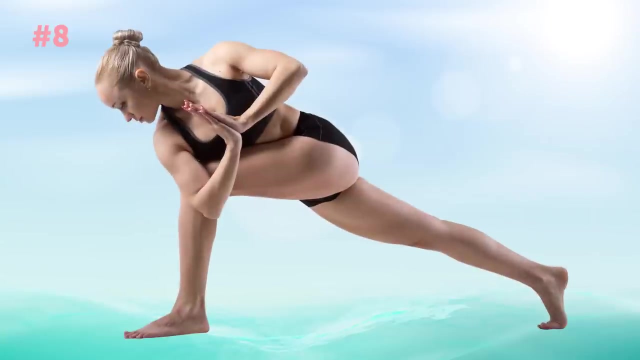 to do it correctly, you need to be able to relax your body fully. don't forget about breathing and sadly, that's all. parivritta parsva konasana. revolved side angle pose. difficult name, but simple asana. kneel into a praying position, stand on one knee and bend. 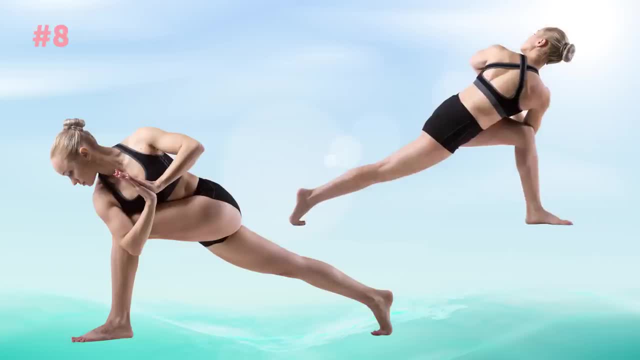 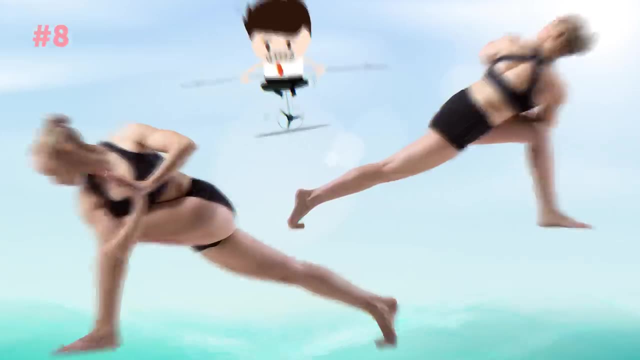 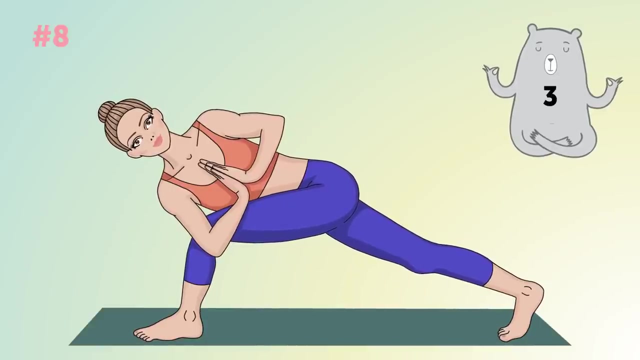 it at a 90-degree angle. then stretch the other leg and balance on your toes. tilt your body to the side. you may even face forward if it helps you keep a better balance. 30-second break on the clock, let's begin. this pose helps strengthen your abdominal core. 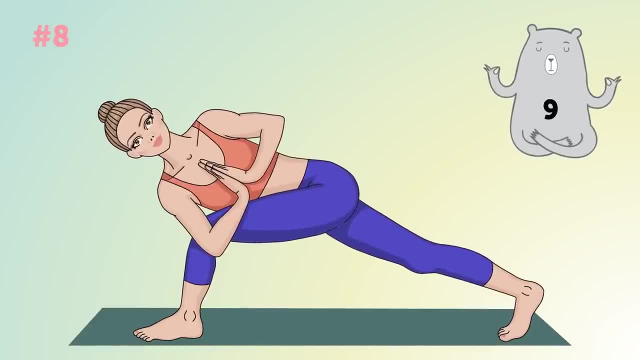 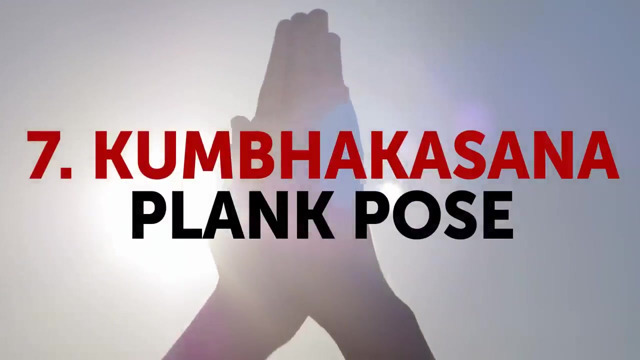 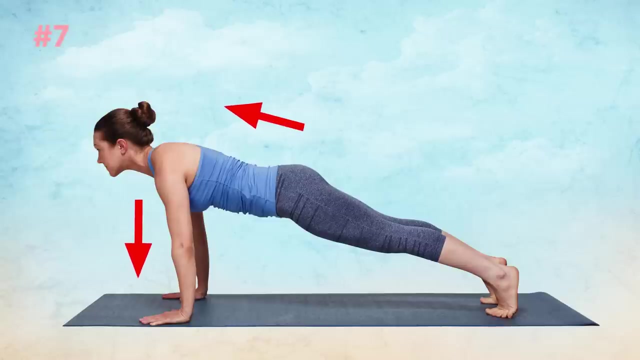 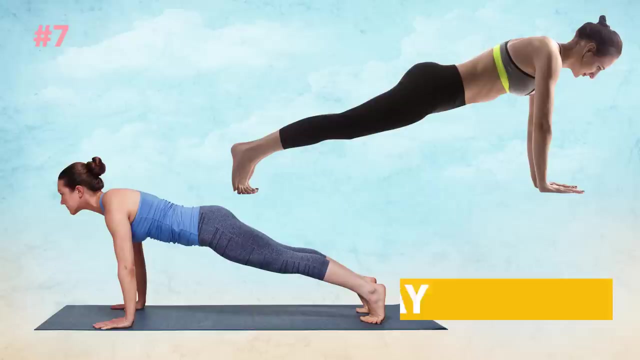 muscles while also stretching your legs, knees, chest, shoulders and ankles. ten more seconds, nice kumbhakasana plank pose. lie face down and lift your body up onto straightened arms, balance on your toes while facing forward or down. we're going to do this pose for 30 seconds, but it's better to extend the time in this pose every day. 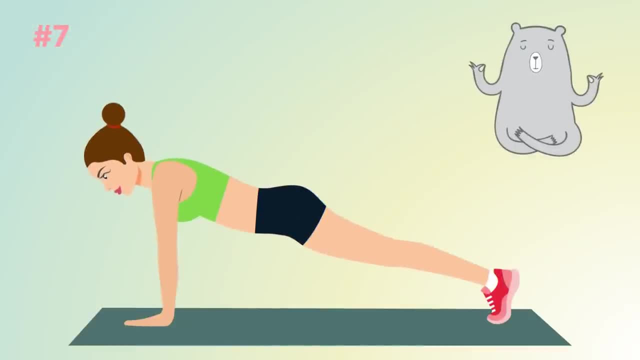 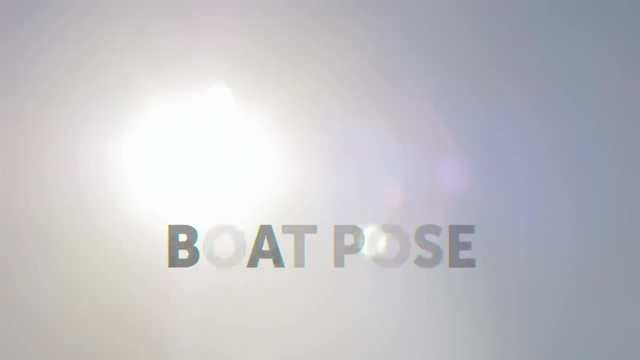 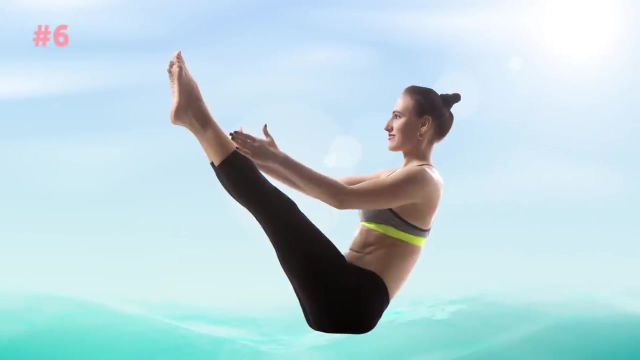 Hold it… Time's up. Paripurna Navasana – Boat Pose. The initial position for boat pose is laying on your back with your legs straight. Slowly lift your legs and your body and stretch your arms by forming sides of the boat. 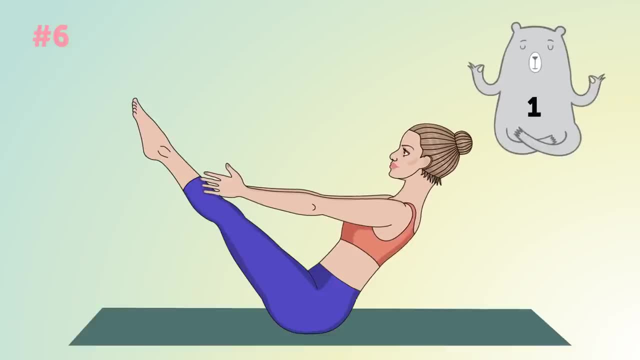 Let's try to hold this pose for one minute. Start the timer. The boat pose will surely work your abdominal muscles, as it cannot be performed correctly without engaging your abs. It also has a positive effect on your digestion and helps you relieve stress. A couple more seconds and you're done. 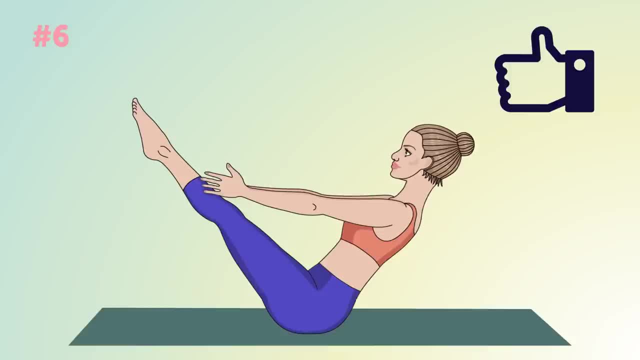 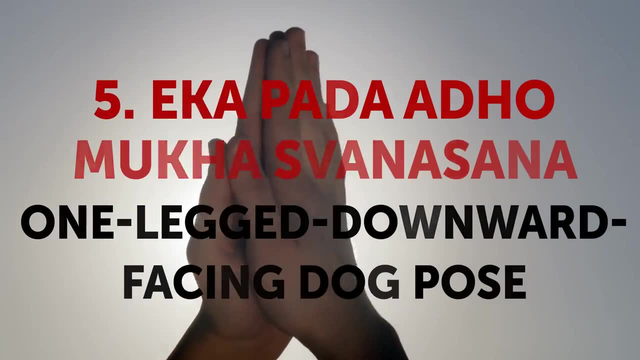 Props to you If you don't break and hold this pose for the entire time. good job, Ekapada Adho Mukha Savasana – One-Legged Downward-Facing Dog Pose. Firstly, get into the downward-facing dog pose. 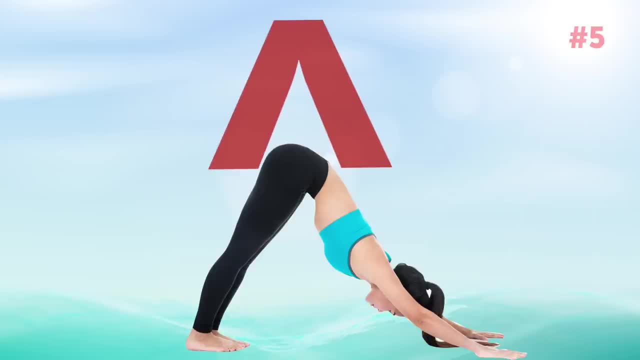 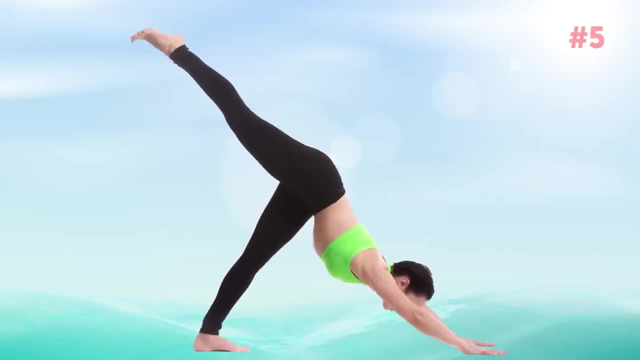 It's an upside-down V-shape that we did a couple of minutes ago. From this position, straighten one leg and lift it up. Then lower the straightened leg under your abs. In one minute. repeat this move 10 times for each leg. 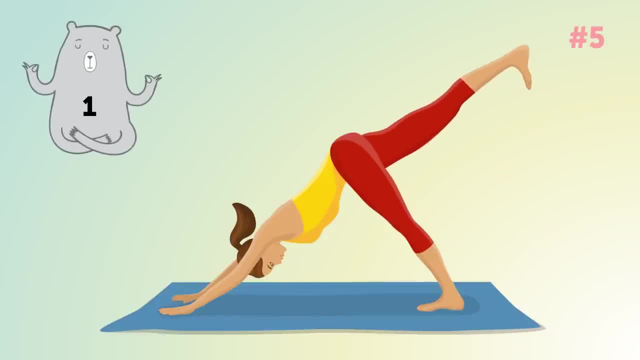 Let's begin. The downward-facing dog pose will help you learn how to balance your body. It can also strengthen your abs. The one-legged version we're doing now stretches your arms as well. It's very easy, isn't it? Let's do it. 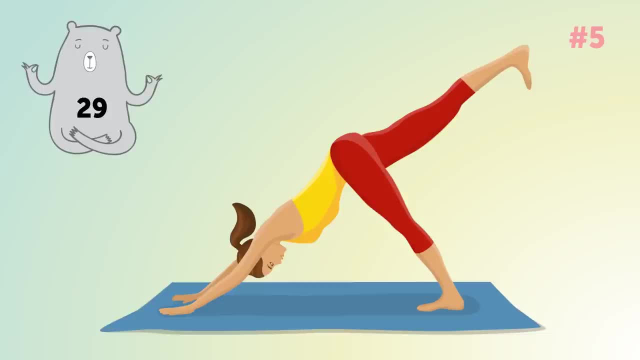 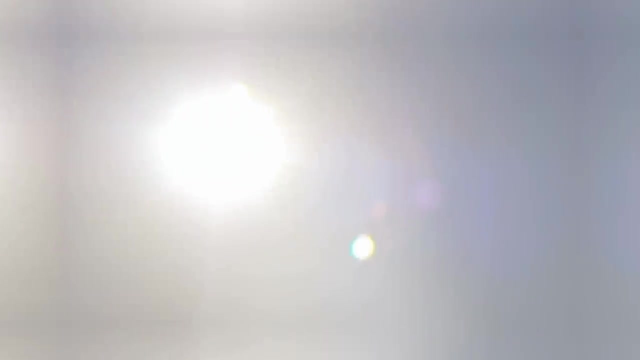 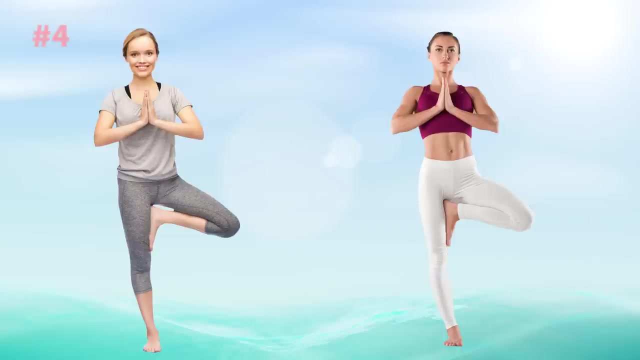 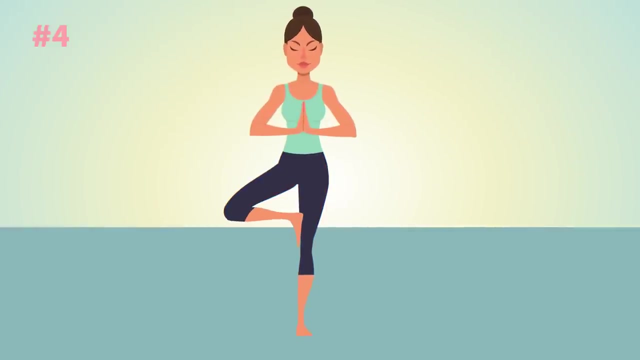 Thank you And finished Triksasana tree pose. Stand up and put your right foot on the inside of your left hip, Put your arms into a praying position And that's a tree pose for you. One minute begins Triksasana tree pose. 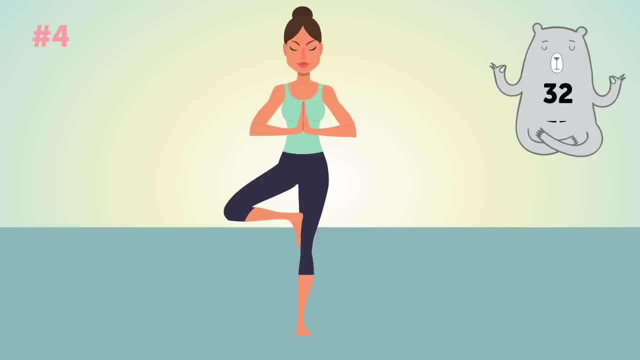 This is another balancing pose that strengthens your abdominal muscles. It is also good for meditation. Just do this pose, Focus on yourself and smile, And you'll see how good it is for clearing your mind And we're done. Dhanurasana bow pose. 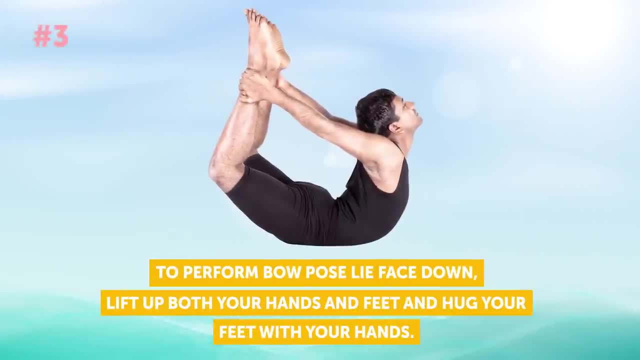 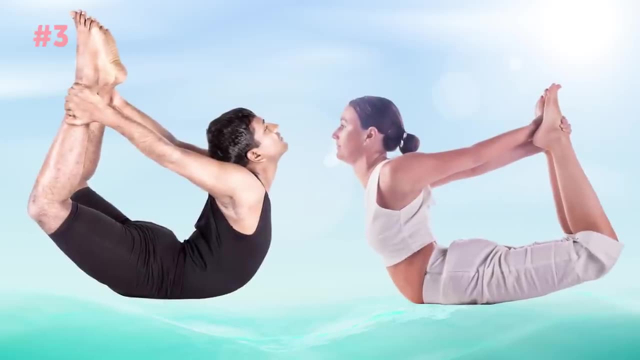 To perform bow pose: lie face down, Lift up both your hands and feet And hug your feet with your hands. We'll hold it for 30 seconds, But as you continue to do this routine in the future, try to hold this pose for at least one minute. 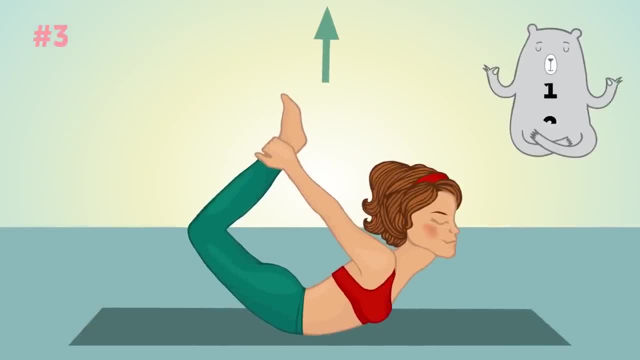 But enough talking, Let's start. The bow pose may look easy to do, but it is the abs that do all the work, which is exactly what you need to strengthen them, A true must-have for the perfectly flat belly. And that's it for the bow pose. 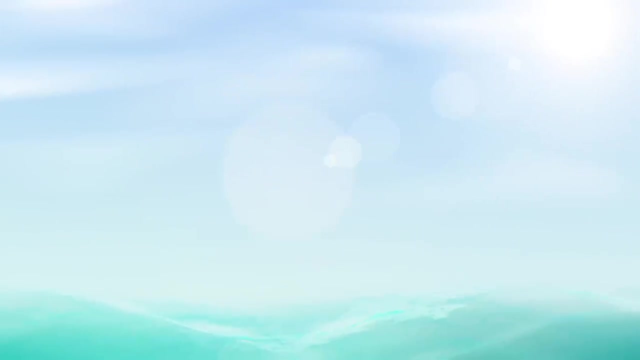 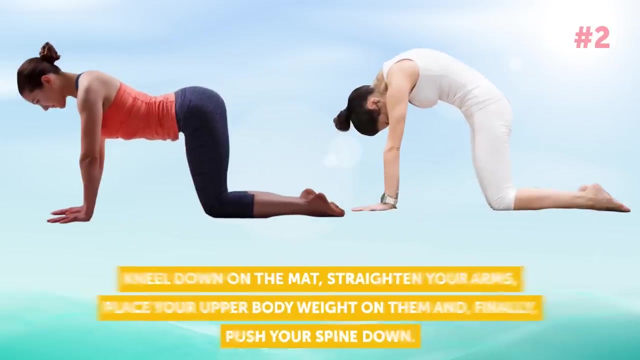 Bittilasana cow pose. Kneel down on the mat, Straighten your arms, Place your upper body weight on them And finally push your spine down. Stay in this position for 30 seconds. Are you ready? 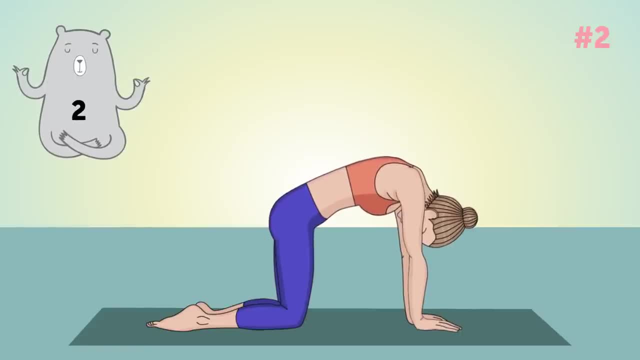 Time to do it. The cow pose is so powerful that daily training can easily make your abs as hard as steel. Sounds cool, right, And we're on our way to it. The cow pose is so powerful that daily training can easily make your abs as hard as steel. 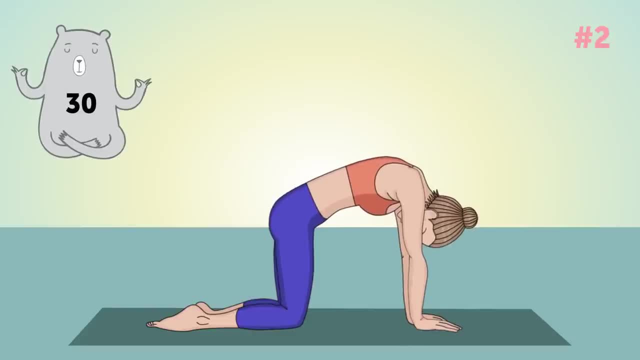 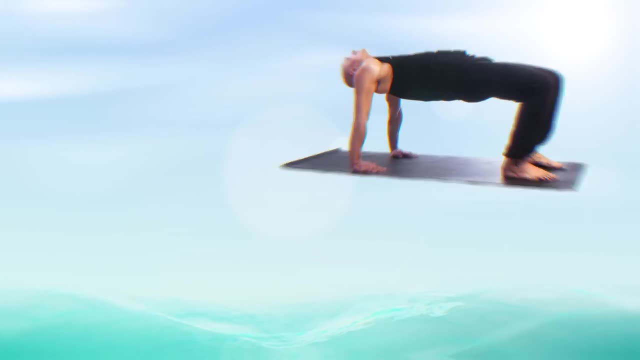 3,, 2,, 1, done. Ardha Purvottanasana- reverse tabletop pose. Sit on the floor with your feet flat and your knees bent In this position. put your arms slightly behind your back, Then lift your arms up. 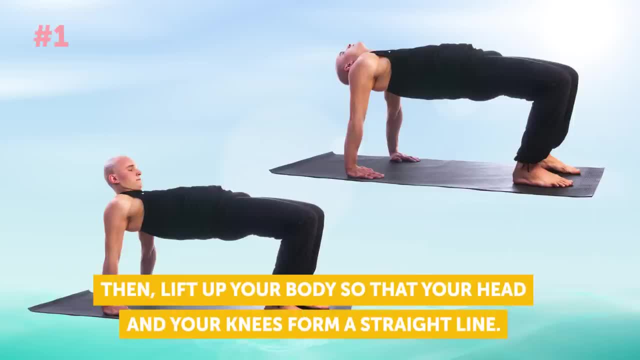 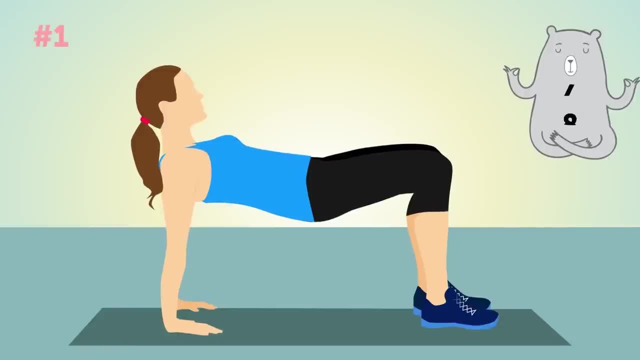 This is an active pose that makes the abs work harder to balance your body. It's especially great for building and toning core muscles and opening your chest and shoulders. And that's the end of our little yoga workout. Come to this video daily and do this workout with us and you won't recognize it.